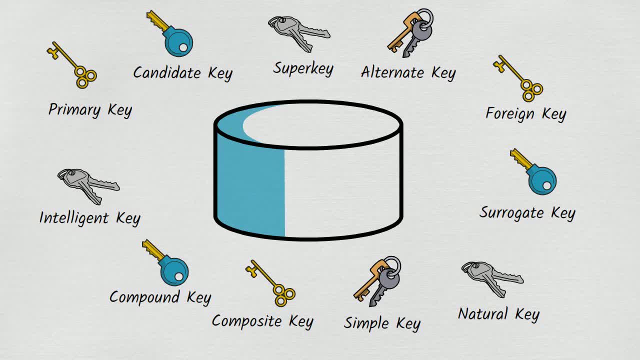 By the end of this video, you'll understand what all this key terminology means, and you'll have gained some insight into how each type of key gets used in practice. This is Decomplexify, bringing a welcome dose of simplicity to complex topics. 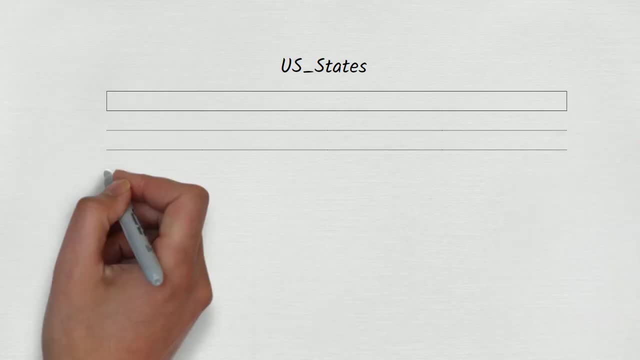 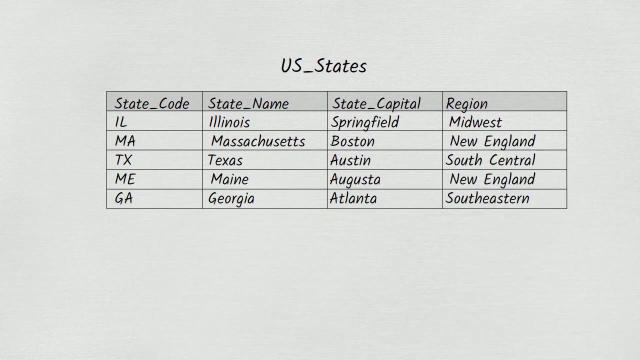 Consider a table called US States. This table contains one row for each US state. Here are some sample rows. Now we ask the question which column of the US States table, or which combination of columns, uniquely identifies a US state? Is it State Code, State Name? 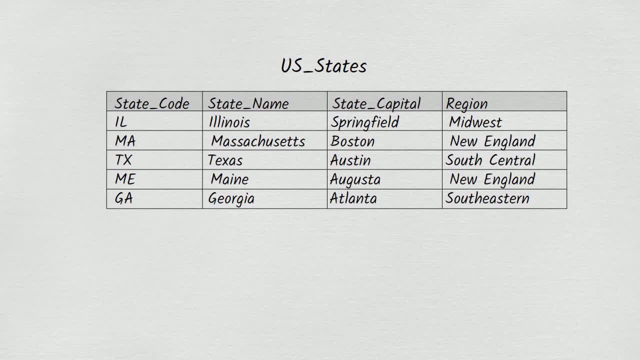 Is it the combination of State Code and Region? Is it something else? Well, we know that a State Code is an official postal abbreviation for a US state. Each State Code officially designates exactly one US state. in real life life, or to put it a different way, state code is a unique identifier for a US state. 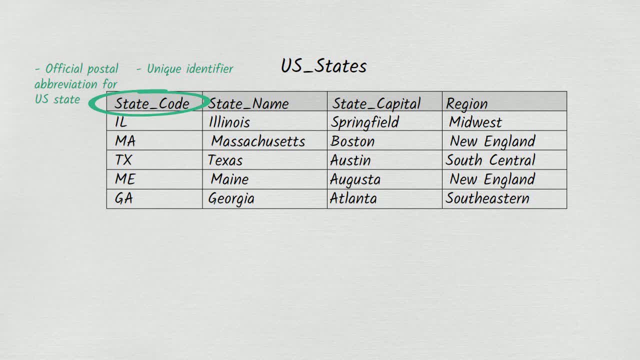 As an identifier, it has one very desirable characteristic – it is highly stable. Stability means that the values of the identifier aren't likely to change their meanings – MA refers to Massachusetts, and we can be confident that we're not going to wake up tomorrow. 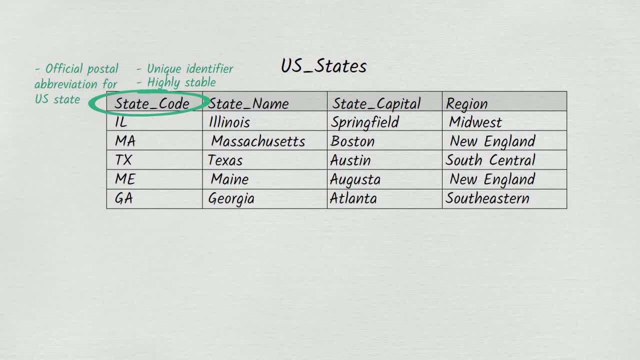 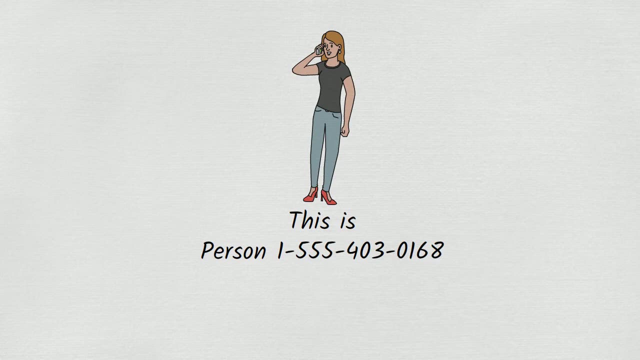 to find that MA now refers to Minnesota instead. But some identifiers don't possess this level of stability. If we were trying to identify people using their mobile phone numbers, we could easily run into problems. A mobile phone number is not a stable identifier for a person, because people can, and quite 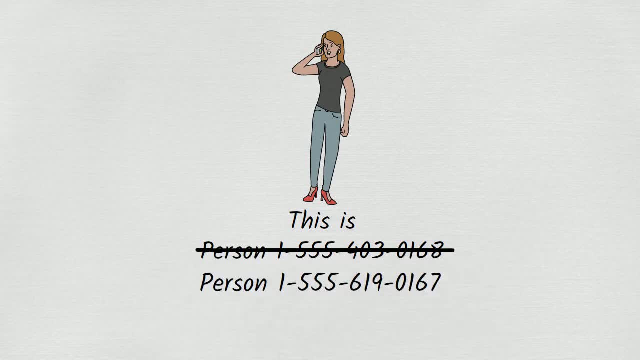 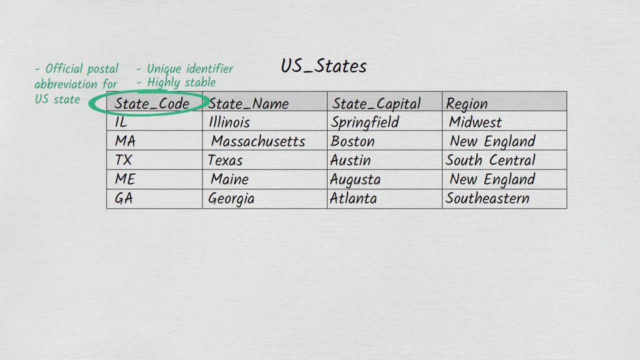 often do change their phone numbers. With state code being a good, stable, unique identifier for a state, we're probably going to want to designate state code as the primary key of the US states table like this. This tells the database platform that the uniqueness of state code needs to be respected. 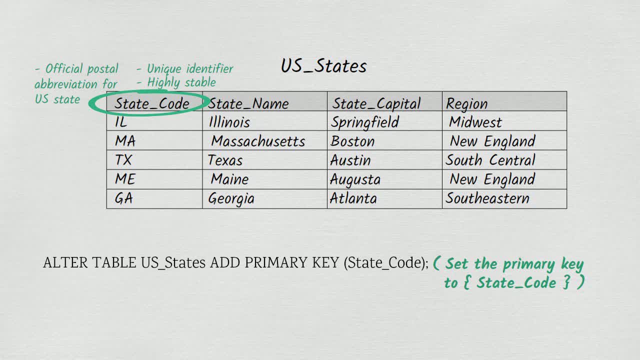 What this means in practice is that if a row currently exists in the US states table with state code TX and somebody tries to insert an additional row with state code TX, then the insert will fail. By making state code the primary key, we're signaling that state code is going to be a 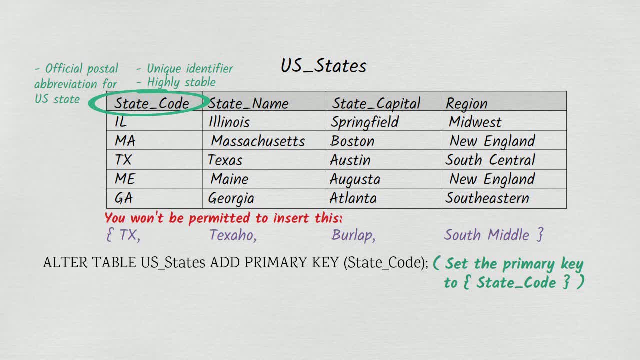 100% reliable shorthand for referring to a specific state, In other words, for referring to a specific row in the US states table. It's also worth mentioning that state code can't contain a null. The database platform doesn't permit you to have primary keys with nullable attributes. 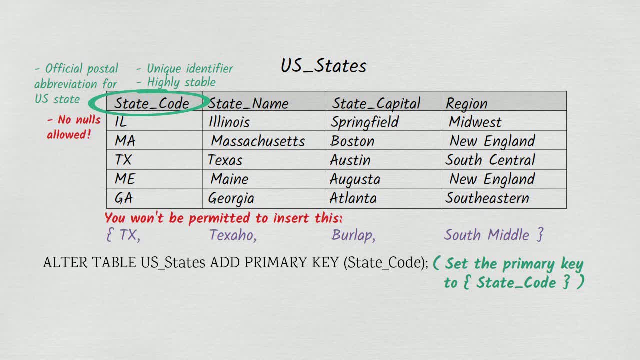 in them. This makes sense because to identify something you need an identifier value, and null isn't a value. Now that the primary key is defined as state code, we can speak of the TX row, secure in the knowledge that there won't be any ambiguity about which row we use. 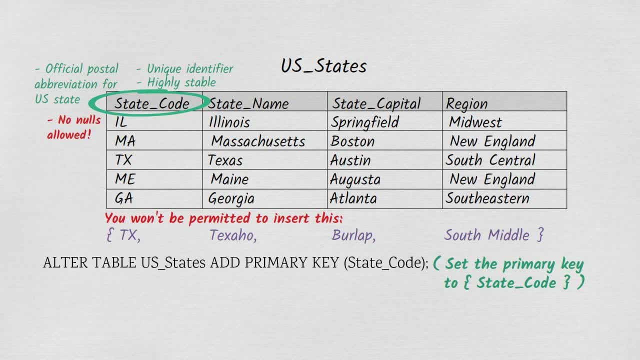 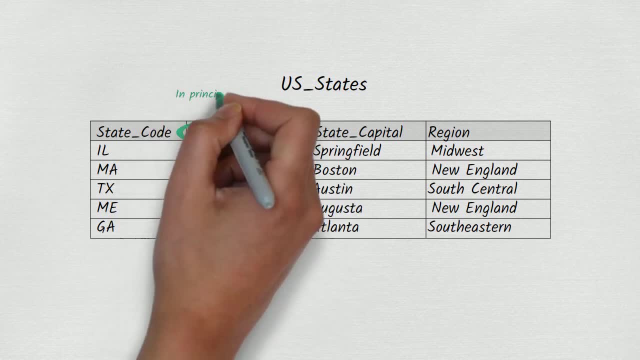 There will only ever be one. Could we have set up the primary key differently? For example, could we have made state name the primary key? Yes, we could have done this, While it's true that geographical entities sometimes share the same name, for instance, 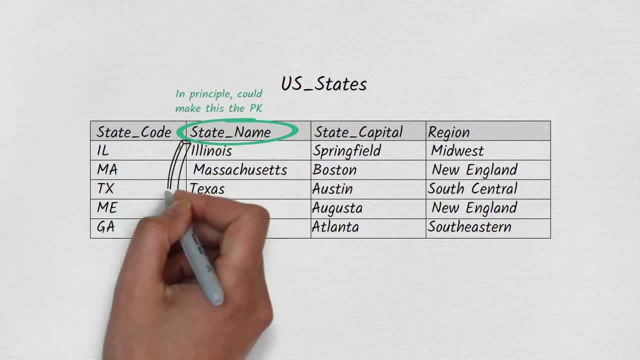 two cities might share the same name, this doesn't apply to US states. All US states have distinct names And even if the US acquires more states in the future, we should be on safe ground in assuming that no US state will ever share the same name. 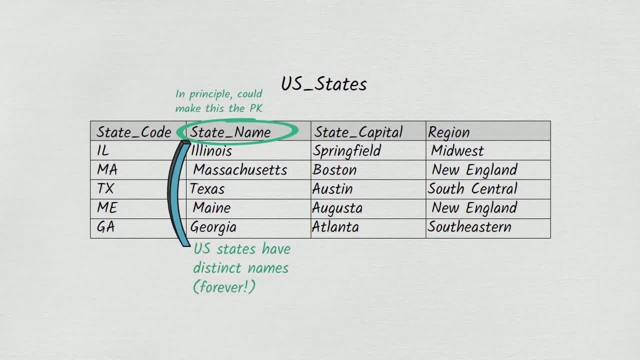 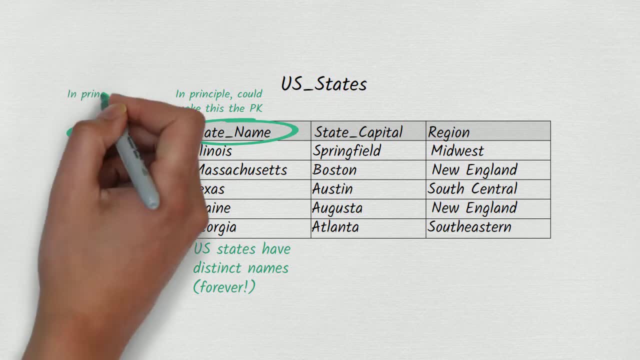 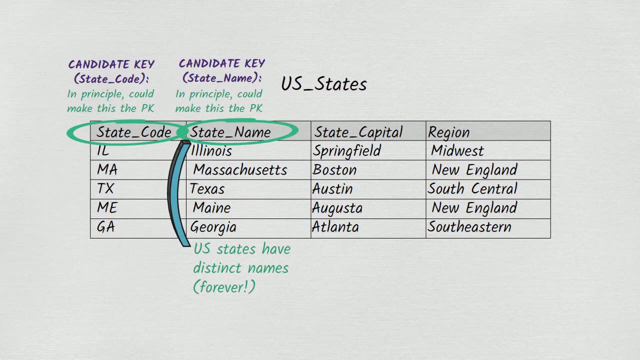 So let's look at some examples. Because state name is a unique identifier, just as state code is a unique identifier, we say that both state code and state name are candidate keys. The term candidate key reflects the fact that when we're deciding what the primary key 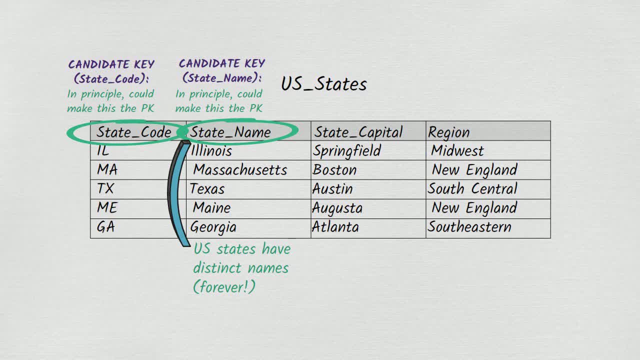 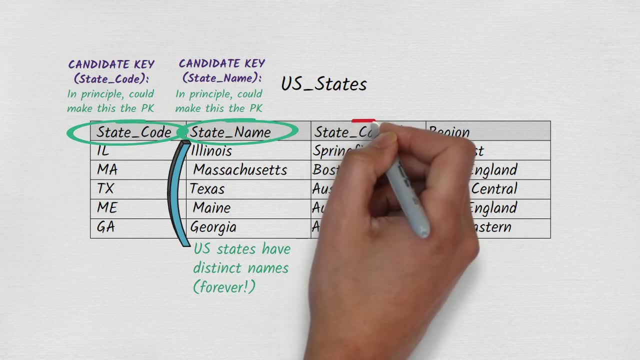 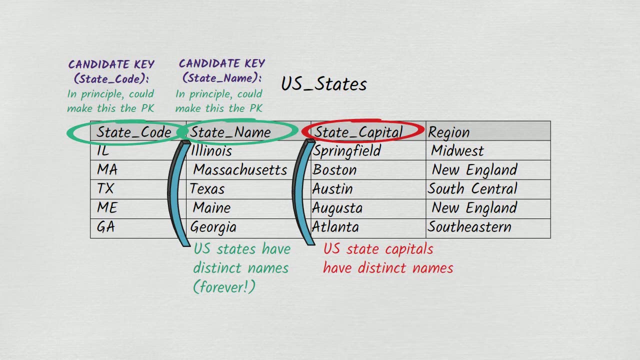 should be. these are the candidates we have to choose from. Are there any other candidate keys besides these two? Is state capital a candidate key for the US states table? We might be misled into believing that it is because no two US state capitals share. 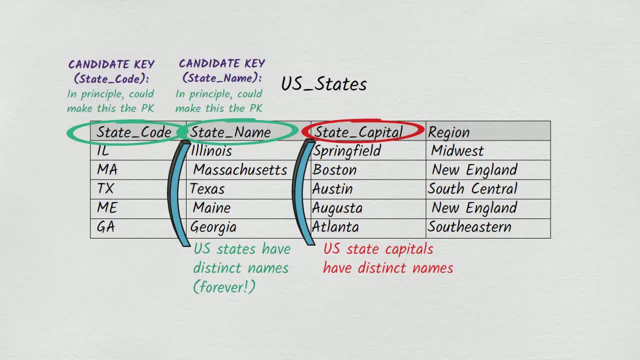 the same name, But the fact that the state capital names are all different from each other is just an accident of history. States have changed their capitals many times in the past and could conceivably do so again – in the latter part of the 18th century, the capital of Georgia was a city called Augusta. 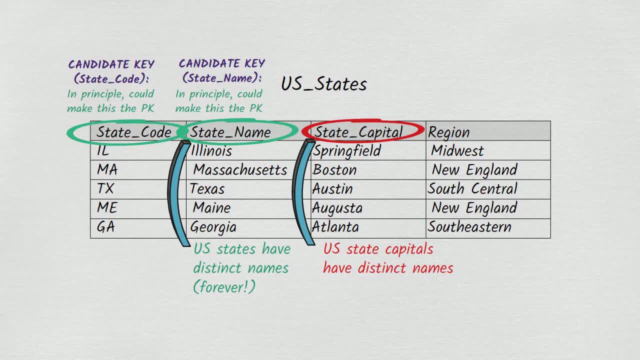 If Georgia changes its capital to Augusta again, then there will be two state capitals called Augusta – the capital of Georgia and the capital of Maine. So state capital isn't a guaranteed unique shorthand for a state – therefore it is not a candidate key. 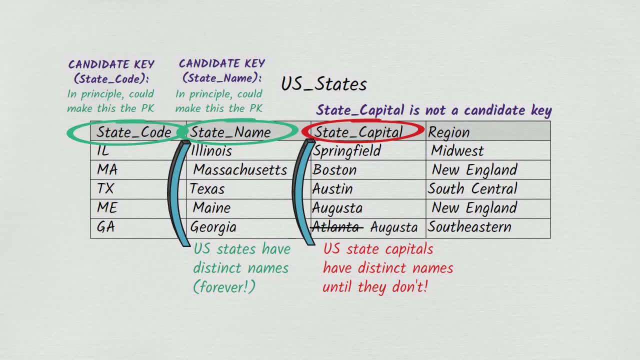 There's a subtle but important point here about what counts as a unique identifier or key. Unique identification isn't just about uniquely identifying things that exist right now. It's about uniquely identifying things across time – even if a certain attribute or a set of attributes seems to act like a unique identifier with respect to things that exist. 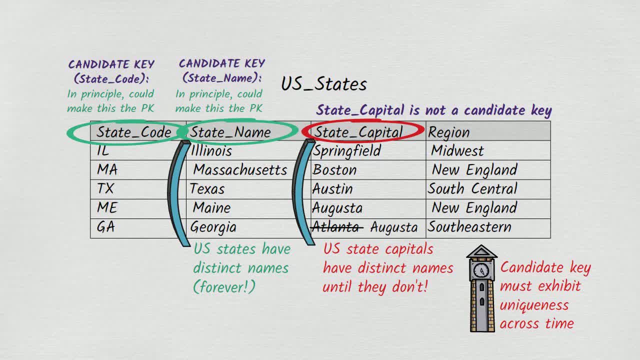 right now. that doesn't mean it can uniquely identify all the things that might exist in the future. For some type of identifier to succeed in uniquely identifying things, we need to be confident that we're never going to come across two of those things that share the 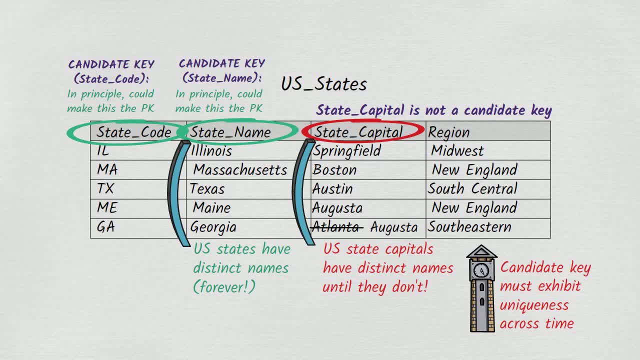 same identifier value – state capital doesn't pass this test. To summarize where we've got to so far in our US states example, There are two candidate keys – state code and state name. State code is probably a better choice of primary key than state name – purely on the 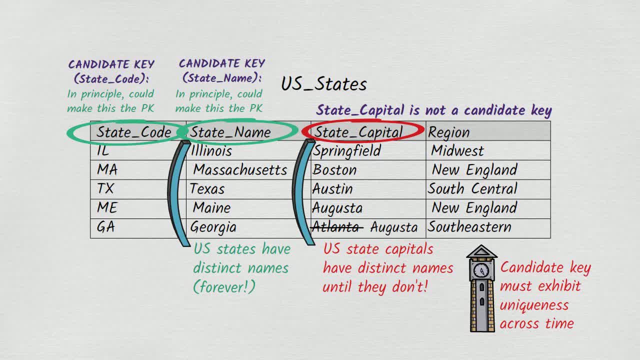 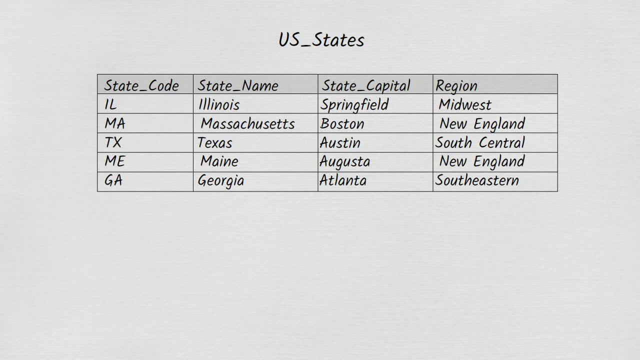 grounds of simplicity – but in principle, either will work. Now let's imagine a database designer who hasn't managed to pin down what the candidate keys are. This designer goes overboard and sets up a primary key that consists of the combination of state code and another attribute. 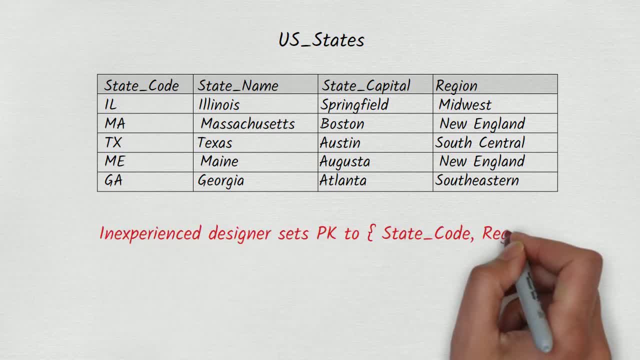 For example, the combination of state code and region, State code and region. Inexperienced designers sometimes have trouble determining which attributes confer uniqueness, and they may end up including too many attributes in the primary key out of a fear that they might otherwise miss out an attribute that needs to be part of the key. 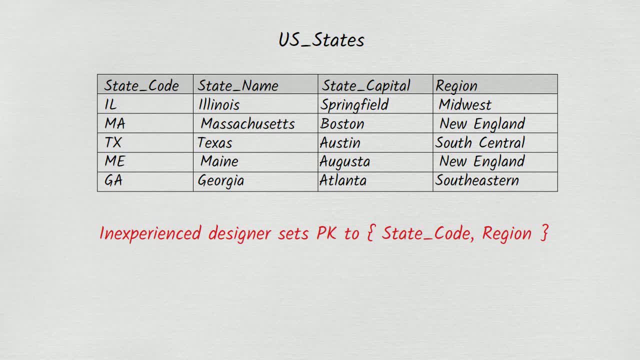 But this is a mistake and just makes things worse. If the primary key is set up as state code region, then the table becomes vulnerable to incorrect data like this: There are now two Georgias, Which is not what we want. The reason this situation has been able to arise is that the primary key the designer. 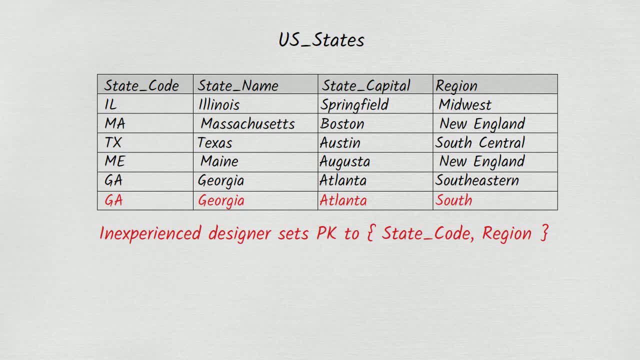 has set up is wrong, And the reason it's wrong is that it isn't irreducible. We call a key irreducible if it has only the attributes it needs to have – in other words, only the attributes that are needed to ensure uniqueness. 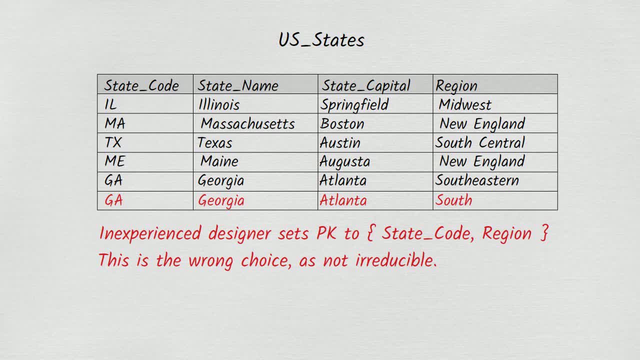 It must not have any attributes besides those, because state code region has an extra attribute that it shouldn't have – namely region. It isn't irreducible, and so it isn't a candidate key. So what can we call state code region? We call it a superkey. 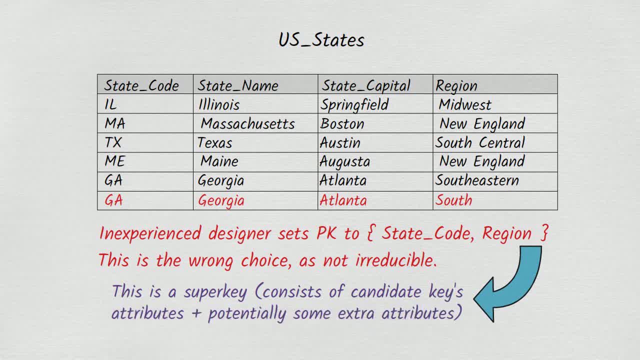 A superkey is something that contains all the attributes of a candidate key plus potentially some additional attributes. You don't normally need to concern yourself too much with superkeys, but the idea of a superkey does show up in theoretically rigorous definitions of the normal forms, as you'll 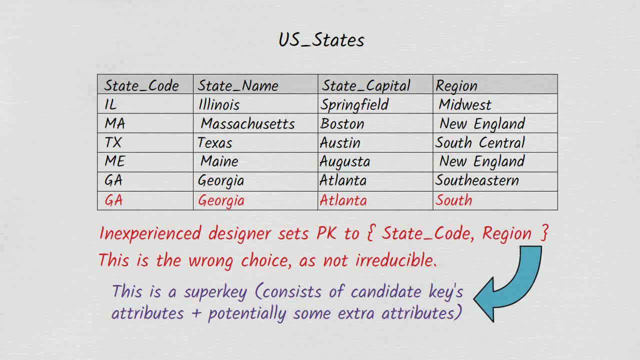 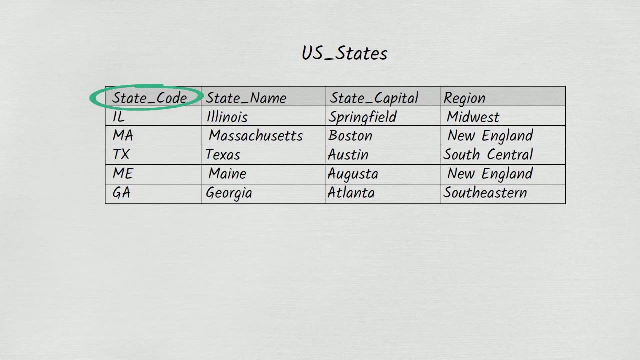 see if you watch Decomplexify's Boy Scouts. There's only one more thing to say about our US States example, and it relates to the fact that the US States table has two candidate keys. We've designated one of those candidate keys- state code- as the primary key, so the 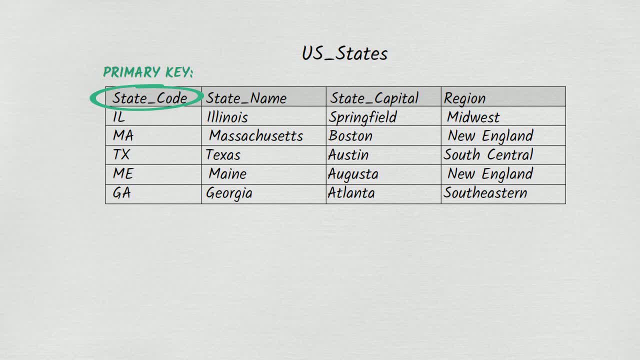 database platform knows it must enforce the uniqueness of state code. But what the database platform won't do, unless we explicitly tell it to, is enforce the uniqueness of the other candidate key: state name. How do we enforce the uniqueness? We can't make state name the primary key, because we've already set up a primary key. 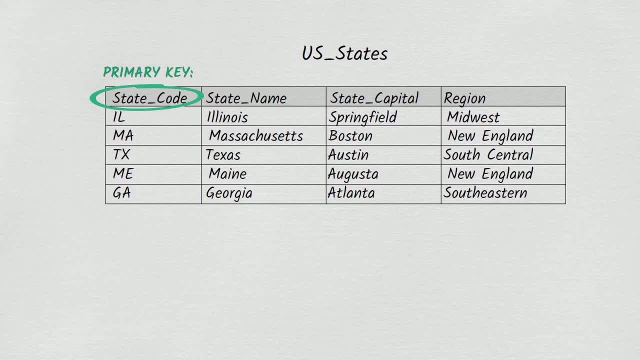 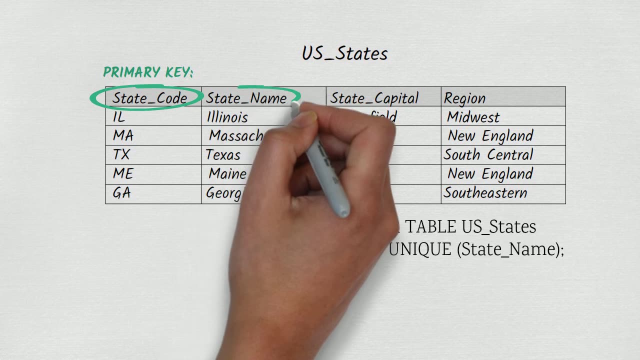 on this table, and having multiple primary keys on a table is never allowed. Instead, we can designate state name as a so-called alternate key like this: By doing this, we're telling the database platform to make sure that the state names within the US States table are all unique. 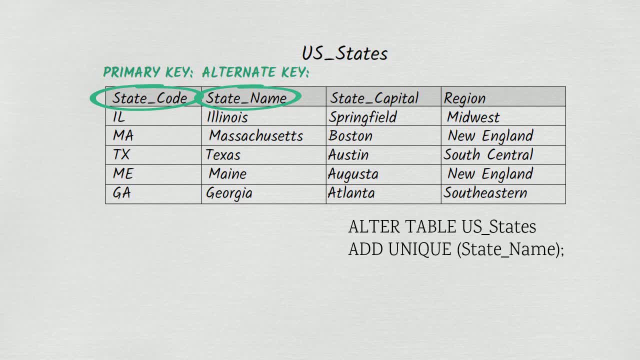 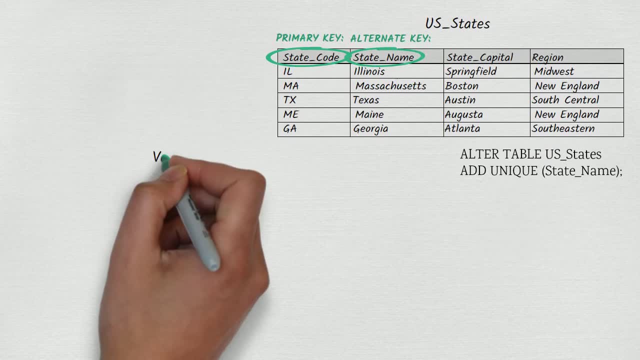 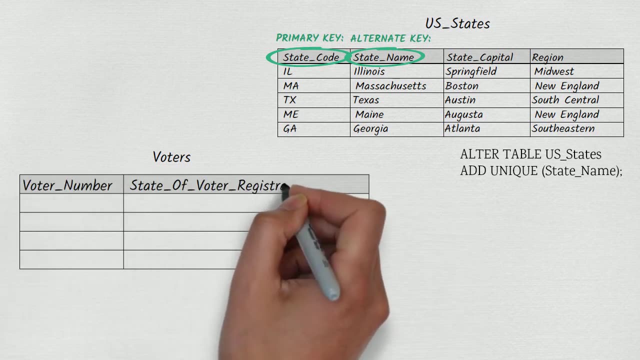 Our database might have other tables besides the US States table that also make reference to US States. Perhaps we have a Voters table that records information about which state a given voter is registered to vote in. Ideally, we want the codes in the State of Voter Registration column to be drawn from. 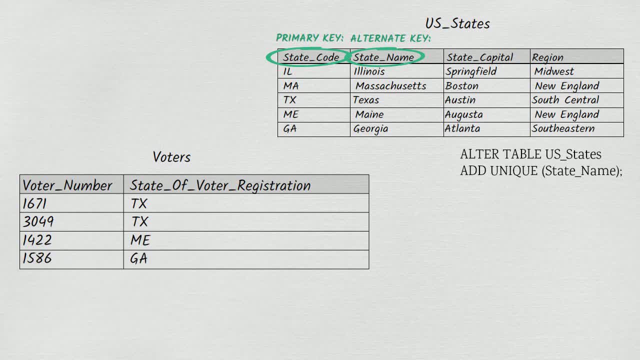 the same set of codes as the ones in the US States table, because otherwise we won't be able to relate one to the other. What state is QX supposed to represent? There isn't a QX in the US States table because there is no US State with a primary key state. 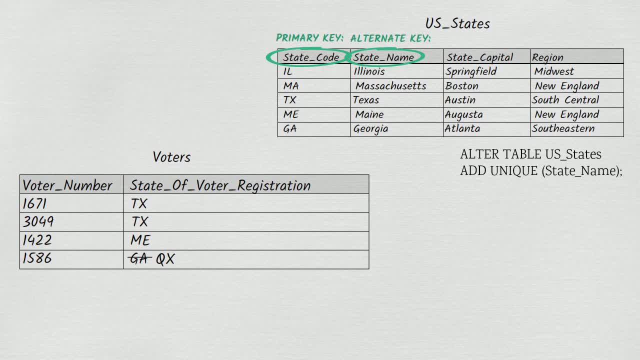 and postal abbreviation QX. It's safe to say QX shouldn't be allowed in the Voters table. so how do we disallow it? The answer is we can set up what we call a foreign key constraint like this: This constraint tells the database that the State of Voter Registration column is a foreign. 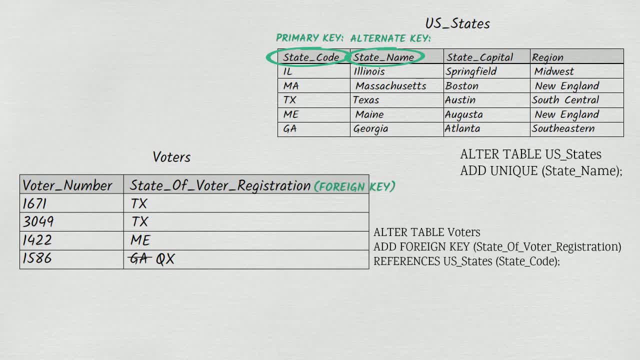 key to the State Code column on the US States table, which means that every value of State of Voter Registration in the Voters table must match a value of State Code in the US States table. With this foreign key in place, State of Voter Registration can never be set to QX because 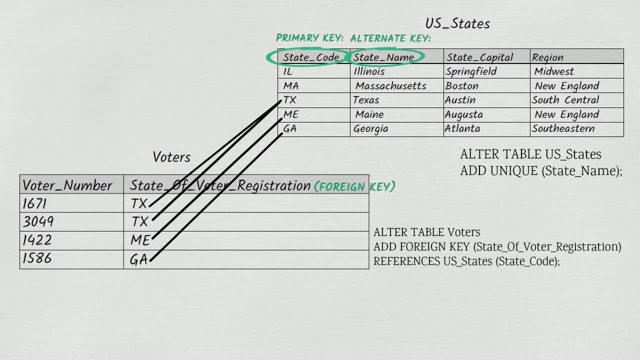 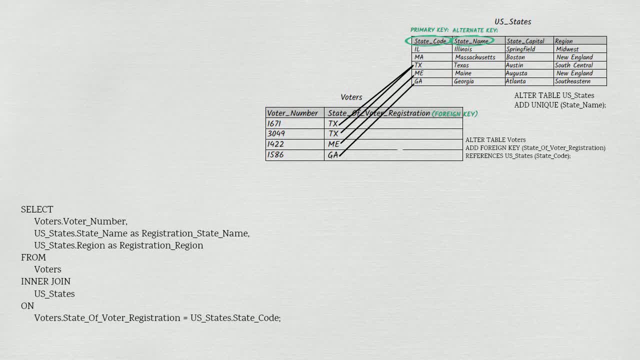 The state from the Voters table equals the state from the US States table and because both these states are expressed using the same convention, namely as US state postal abbreviations like TX and GA, our join should give the desired results, Interestingly from the point of view of being able to join the Voters table to the US States. 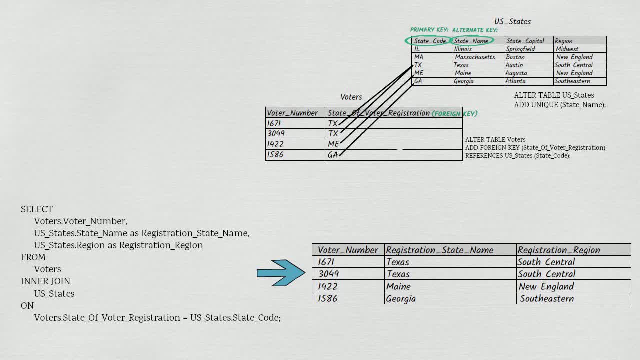 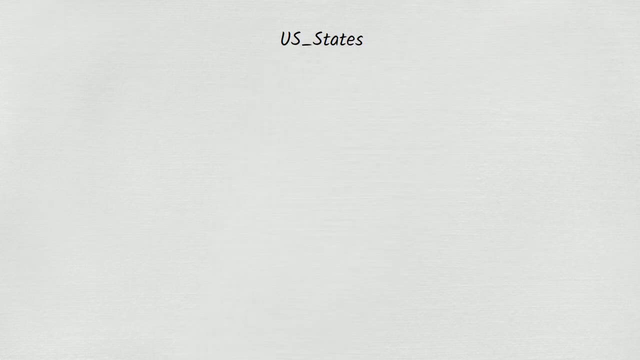 table. it really doesn't matter if the states get represented as meaningful State Codes like GA or as completely arbitrary codes that we've fabricated ourselves For the purposes of this particular database. we could have gone for an alternative design, where each state has an arbitrarily assigned numeric State ID, like this: 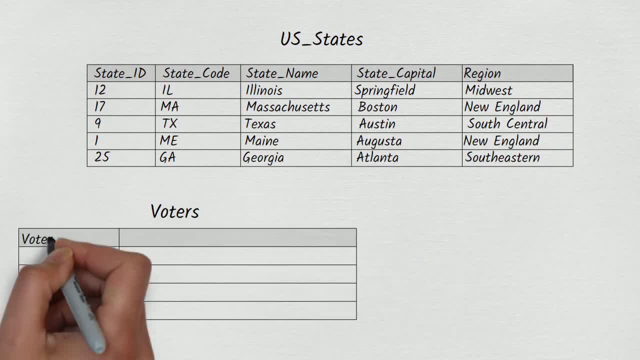 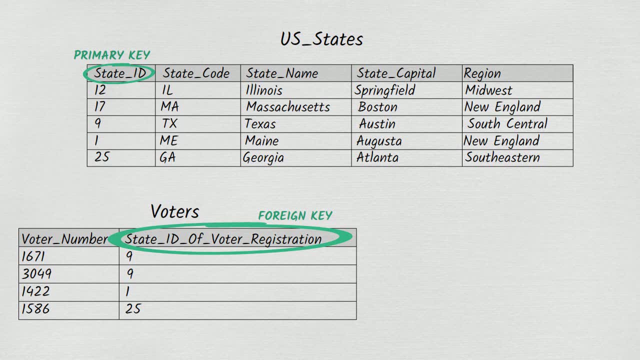 In the alternative design, State ID is the primary key of the US States table and State ID of voter registration is a foreign key on the Voters table. If we want to join the Voters table to the US States table, our query looks much as it. 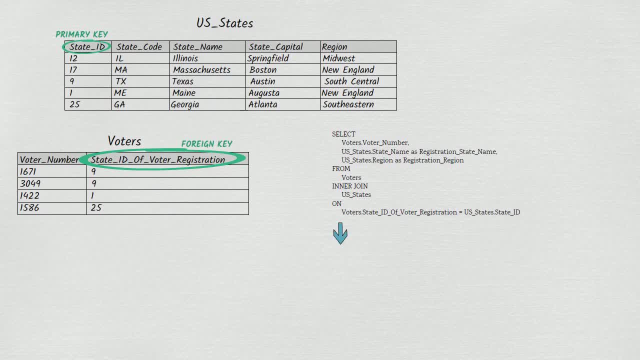 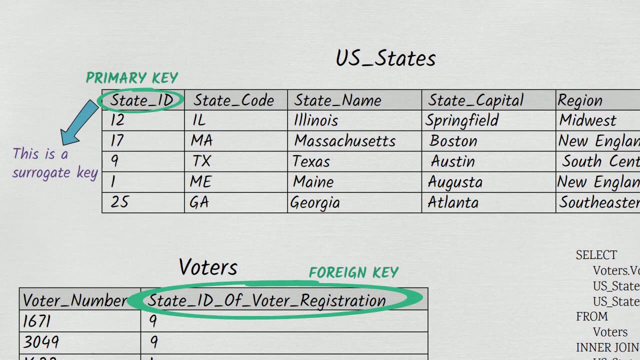 did before, except this time we joined the Voters table to the US States table. The output of the query is exactly the same as before. State ID in this example is what is known as a surrogate key. A surrogate is a thing that stands in for something else. so, for example, in our alternative: 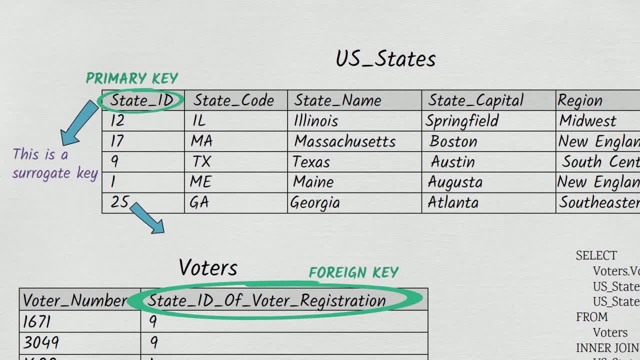 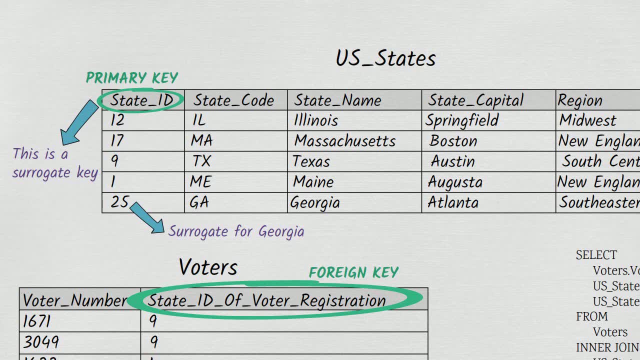 design State ID. 25 is a stand-in for GA or Georgia. One big difference between 25 and GA is that lots of people in the real world are familiar with GA as a shorthand for Georgia, whereas nobody in the real world associates 25 with 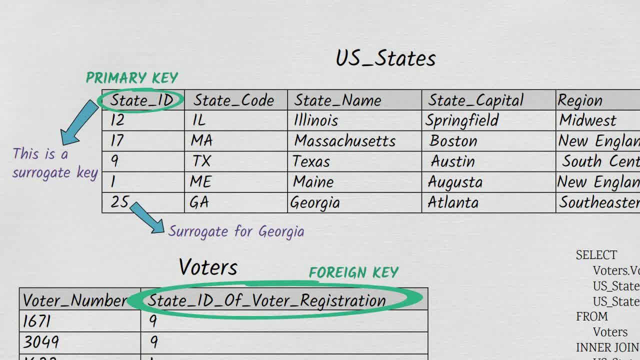 Georgia 25 only means Georgia in the context of our database, And that's the essence of a surrogate key. The surrogate key's values only have real-world meaning within the context of our database. If we're using the term surrogate key to describe the State ID in the alternative design, we 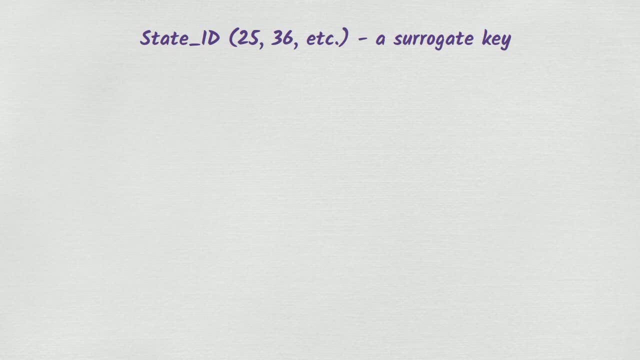 need a term to describe the state code from the original design. We refer to the state code from the original design as a natural key, because its values – GA, TX and so on – are the values that a person would naturally, as it were, use. 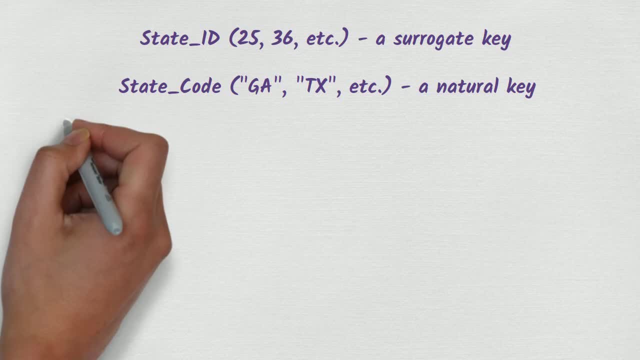 in real life to refer to US states, for example, when writing an address on an envelope. Just as we can have a natural key representing a state, we can have a natural key representing a person. Many countries have some form of national ID – a national insurance number. in the United, 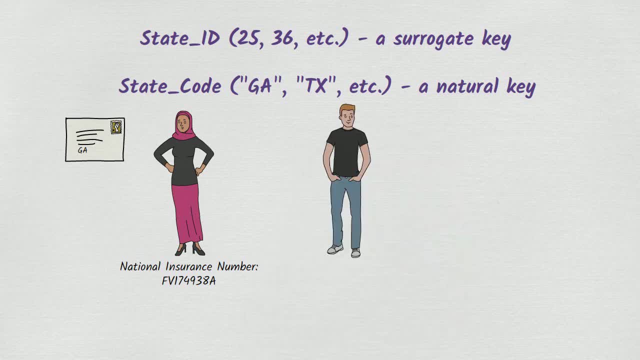 Kingdom, for instance, or a social security number in the United States, These identifiers would qualify as natural keys. An email address is a natural key. If your insurance company sends you a letter which has your customer number at the top of it, this customer number is a natural key. 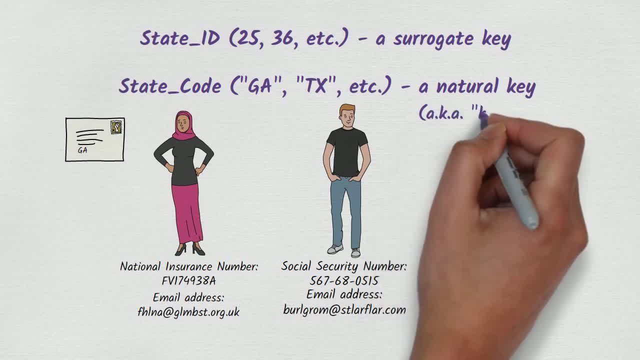 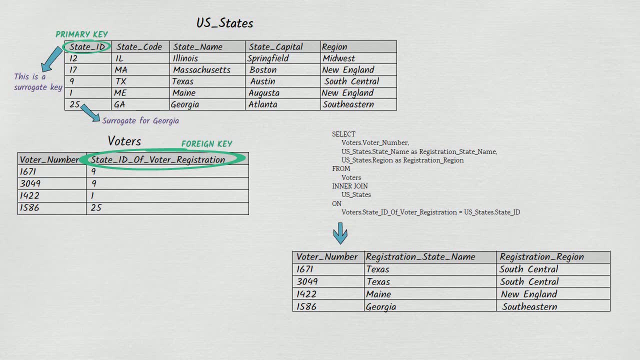 And it's worth noting that natural keys are also sometimes known as business keys. Surrogate keys are different. The meaning of any particular surrogate key value isn't something that gets shared with the public. The way we decide which surrogate key values within the database represent which real-world 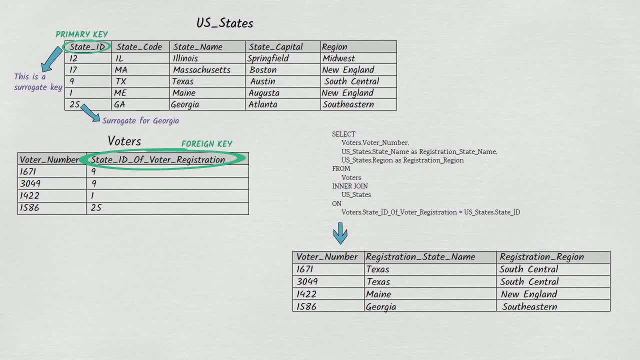 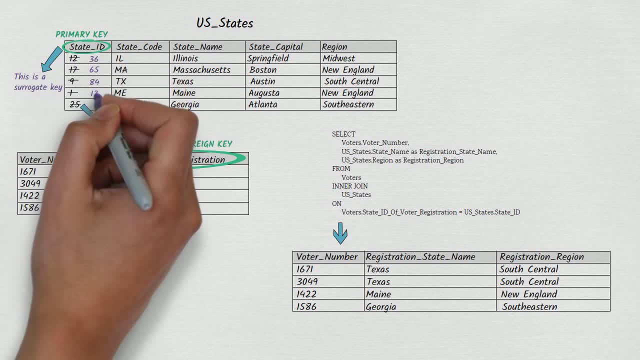 things – for example, which state IDs represent which states – is arbitrary, Even if every single surrogate key value in the database changed overnight, which, let's be clear, wouldn't happen. but even if it did, then as long as those key values changed. 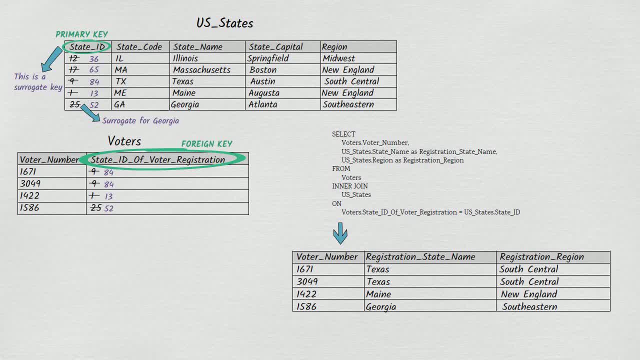 in a completely consistent manner, everything would work exactly as it did before. Surrogate keys have a crucial role to play in database design, But trouble arises when we forget that each surrogate key value has to represent one very specific thing in the world. The job of a surrogate key is not merely to identify a record or row. 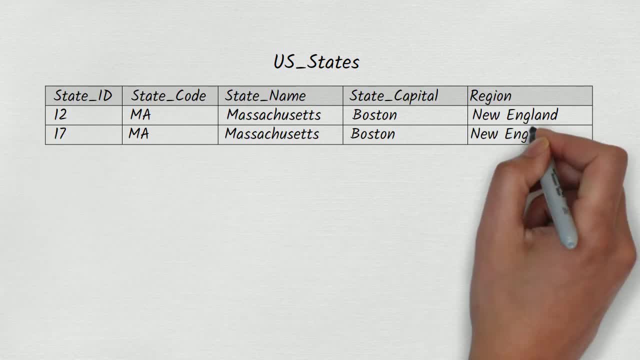 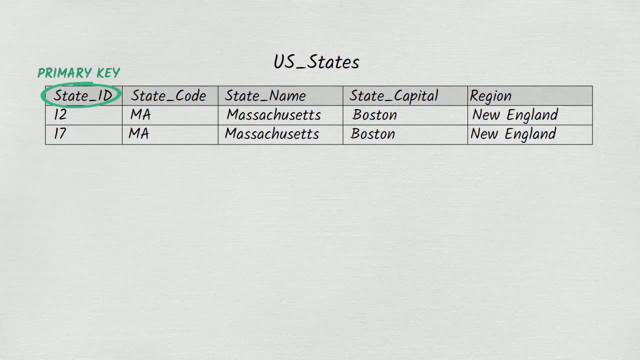 If a surrogate key were just a row ID, then this could happen. These two rows are distinct from each other because they have different state IDs, But what's the point of that? Both rows are clearly about Massachusetts, whereas what we really want is for all the. 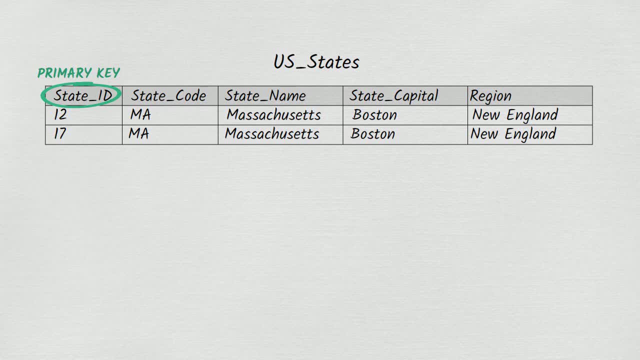 state IDs in the US States table to refer to different states. In this case we could resolve the problem by setting up state code as an alternate key, which would ensure that we never get multiple state IDs referring to the same state. In other situations there might not be a suitable alternate key available, but at the 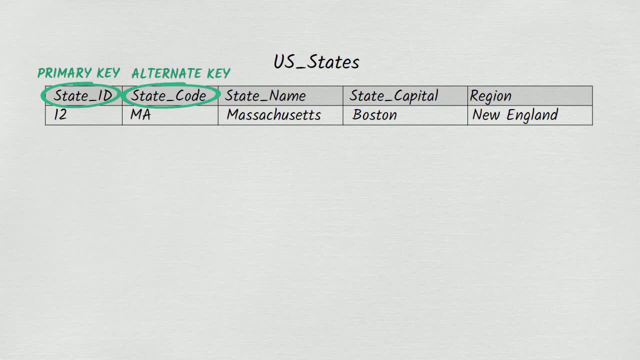 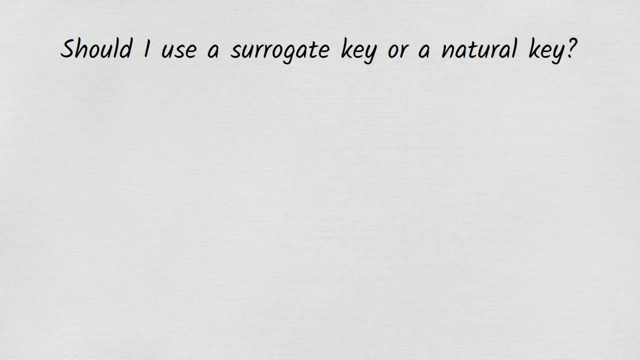 very least, we should ensure that the process that inserts records into the table takes care to avoid inserting multiple records that refer to the same thing. in the real world, If you're a database designer, you'll often be faced with the decision of whether to implement a surrogate key or a natural key. 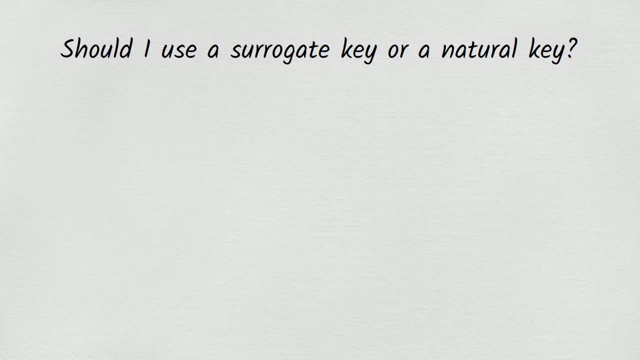 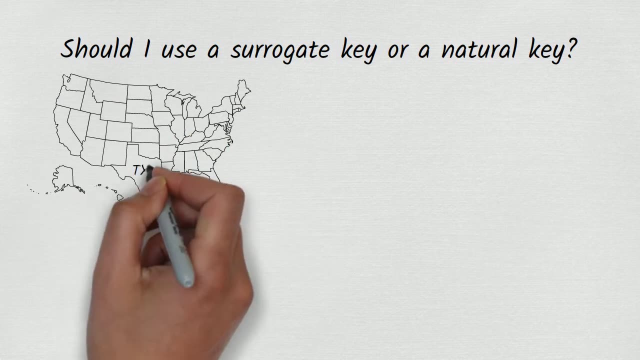 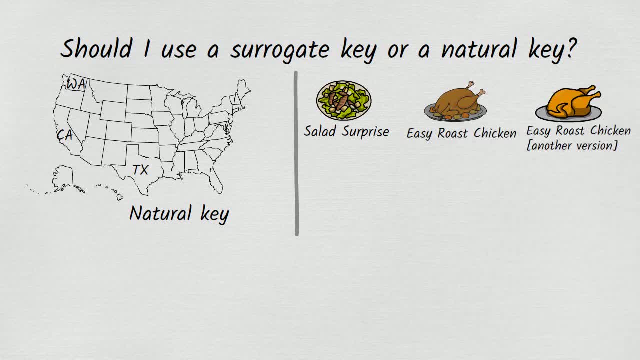 What natural key could we use to uniquely identify a recipe? There aren't really any good options, so a surrogate key is probably a sensible choice for identifying a row in a recipe table. In still other cases a real-world unique identifier exists, but there are limits to. 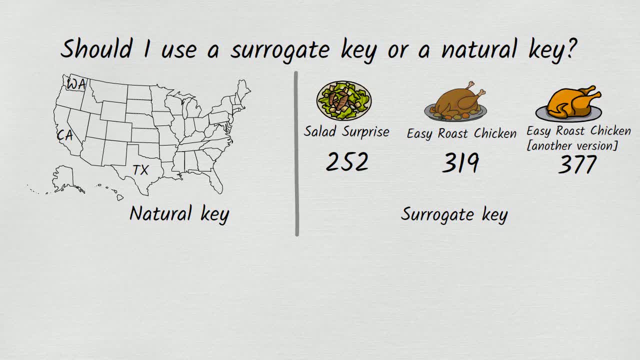 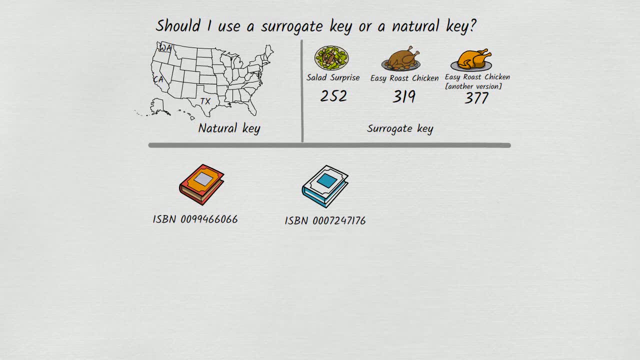 its scope, which mean it wouldn't be a suitable primary key. For example, an ISBN number is an internationally recognized numeric code for identifying books. It is a natural key. Let's say we're an online bookseller and in our backend database we have a books table. 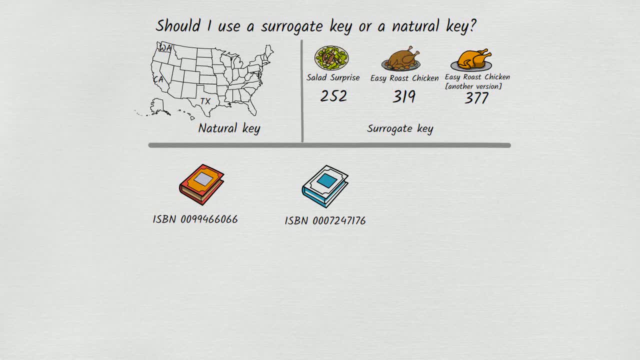 We might be tempted to use the ISBN as the primary key of the books table, But if the books table is supposed to include ebooks as well as print books, then ISBN turns out not to be a suitable key, Because the reality is that lots of ebooks don't have an ISBN number. 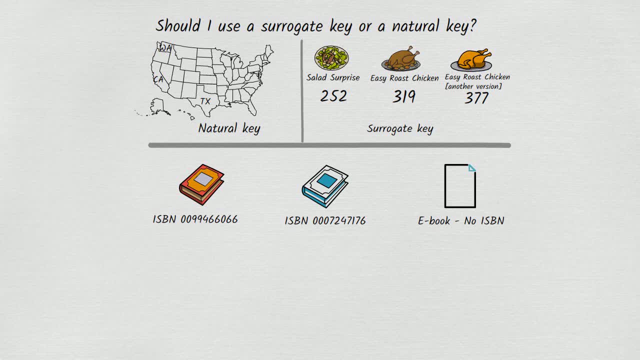 Instead, we are better off inventing our own book numbers, which apply to ebooks as well as print books. These book numbers will be contained in a column called book number, which will be the primary key of the books table. ISBN is still a useful piece of information, so we'll still have an ISBN attribute in 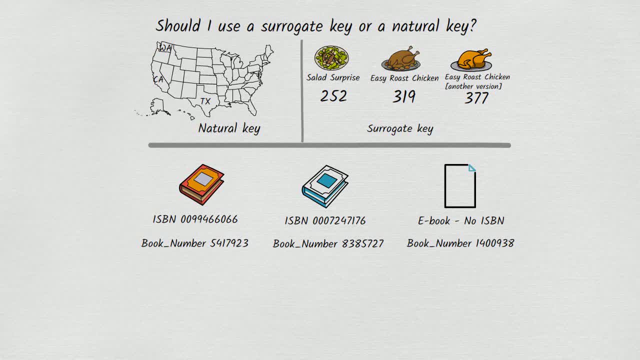 our database, it just won't be the primary key. As for book number, we might ask: is it a surrogate key? Well, it is a surrogate key if we ensure that the book numbers aren't publicized, But if we make the book numbers visible to the public, for example by displaying them. 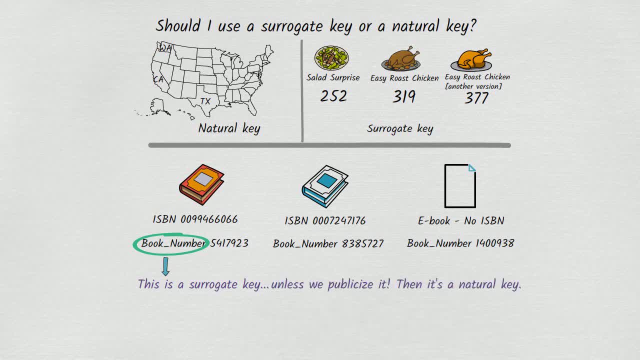 on the product page, then we can make sure that the book numbers are not publicized. So if we select the product pages of our company's website, then book number becomes a natural key. One thing you may have noticed is that in most of our examples so far, the primary key 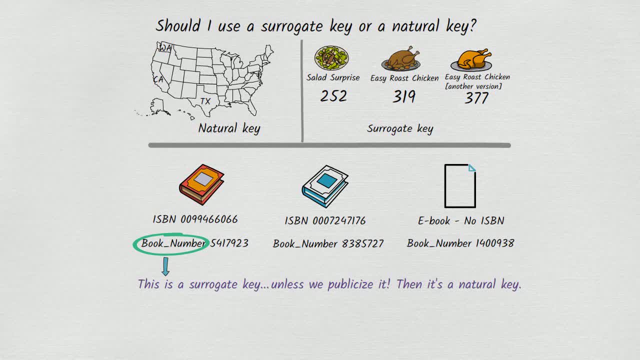 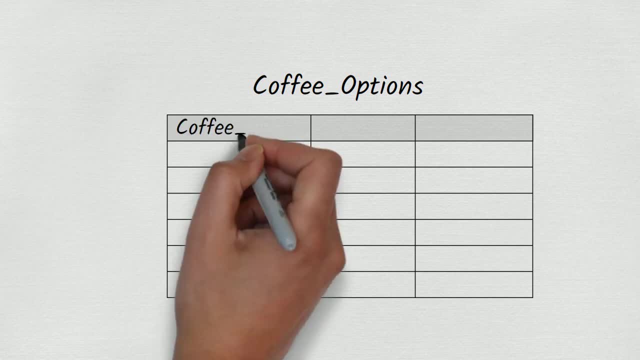 has consisted of a single column. This doesn't have to be the case. We might have a table that gives the prices of different coffee options in a cafe. Clearly, a coffee option in this table is uniquely identified by the combination of coffee type and cup size. 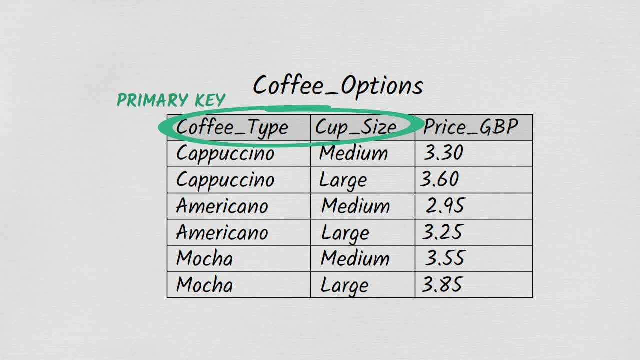 So we can designate the primary key as coffee type cup size. We call a key composite if it consists of more than one attribute, so coffee type cup size is a composite key. If a key consists of just one attribute, we call it a simple key. When we have a composite primary key, any foreign key that references this primary key will also be composite. For example, if we have a table that records each person's preferred coffee option, it will look like this: On this table, which has primary key person, we define a foreign key coffee. type of preferred option. cup size of preferred option. 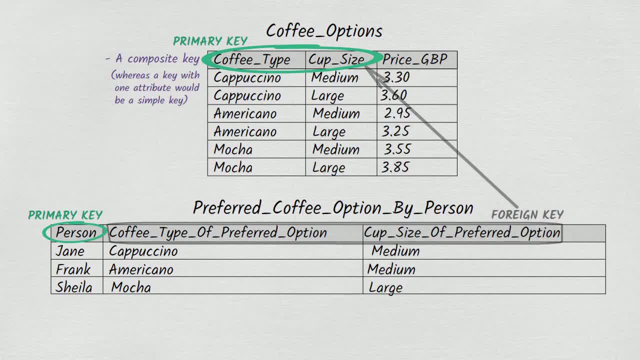 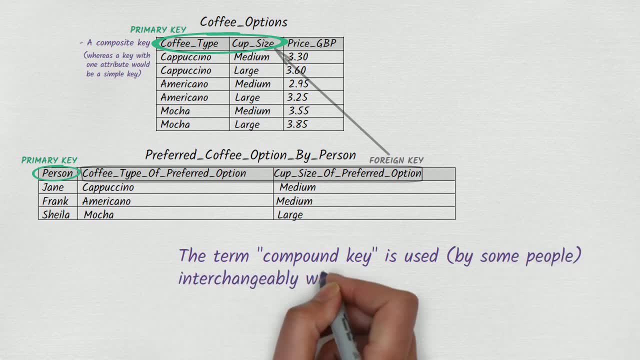 which references the primary key coffee type cup size on the coffee options table. It's worth mentioning that some people use the term compound key interchangeably with the term composite key. Other people only say compound key when they mean a particular type of composite key. 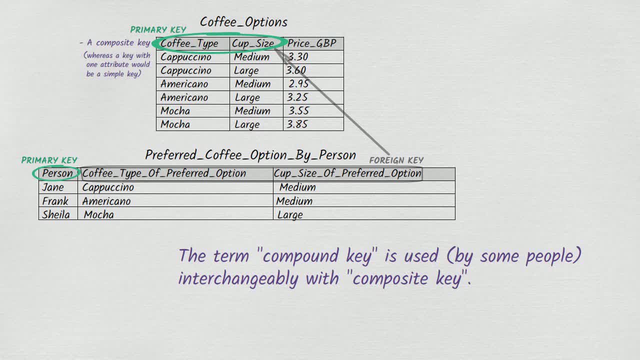 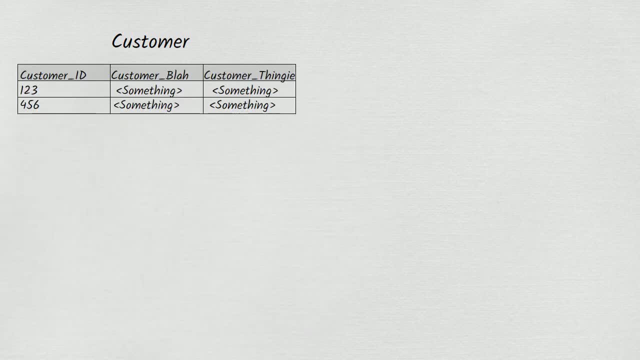 namely a composite key that contains at least one attribute, That's a foreign key to some other table. For example, if we have customers and accounts and each customer can have multiple accounts and vice versa, then we're probably going to have a customer table, an account table and a. 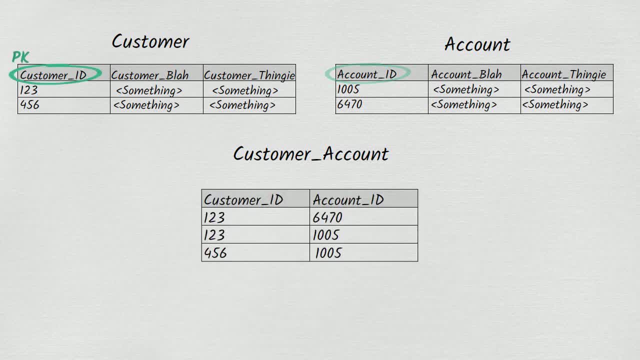 customer account table that shows the linkages between specific customers and specific accounts. like this: The primary key of the customer account table is customer ID, account ID. Customer ID is also a key to the customer account table. Customer ID is also a foreign key to the customer table. 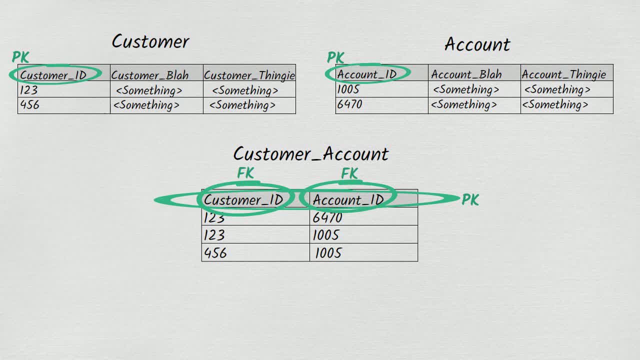 An account ID is a foreign key to the account table. The primary key of the customer account table has two attributes that are both foreign keys, So it is a compound key in this sense. The last term we're going to look at is the term intelligent key. 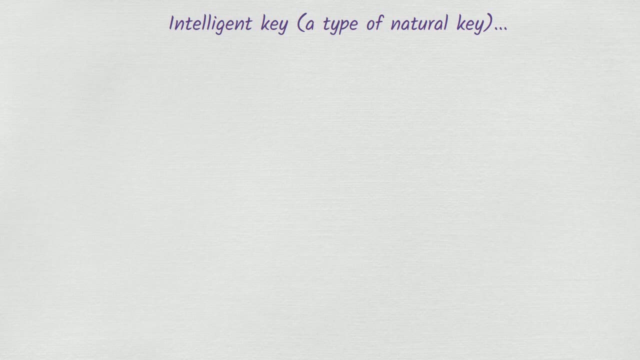 An intelligent key is a particular type of natural key. Let's suppose we're a company that makes children's toys. We have a standard way of classifying the toys that we produce At a high level. we have two product categories: classic and modern. 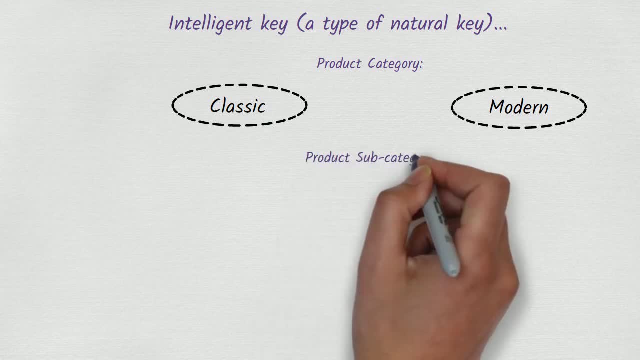 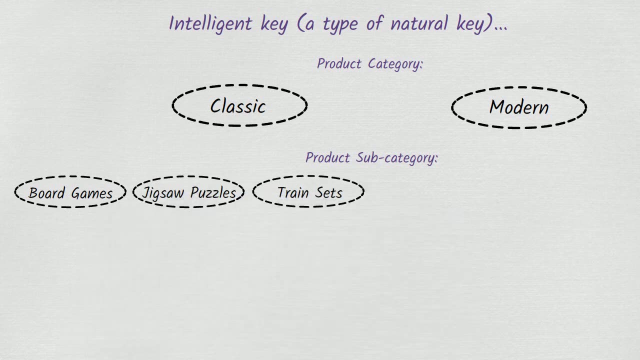 Each product category is subdivided into product subcategories. The classic category has three product subcategories: board games, jigsaw puzzles and train sets. The modern category has two product subcategories: quadcopters and sentient teddy bears. And finally, within each product subcategory, we have individual products, each represented by a product code. 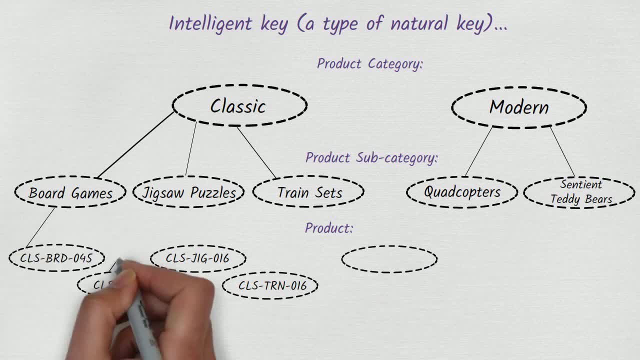 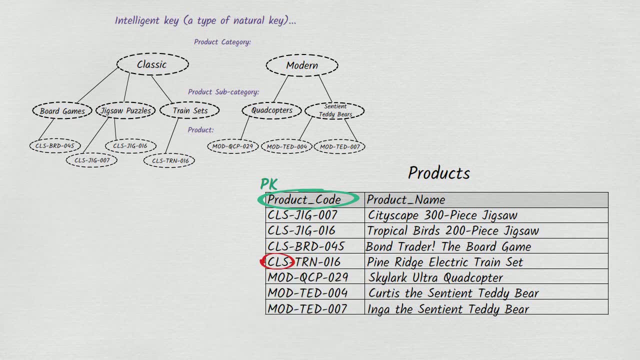 Notice the format. The product code is composed of three parts. The first part represents the product category- classic or modern. The second part represents the product subcategory, like jig for jigsaw or QCP for quadcopter, And the third part is a sequence number that denotes the specific product within that subcategory. 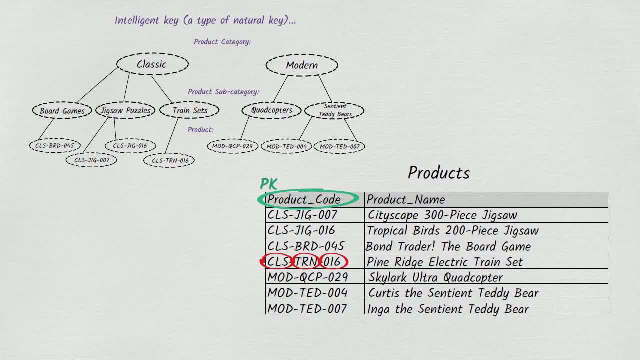 So, for example, the Pine Ridge electric train set has product code CLS-TRN016.. The CLS part means classic and the TRN part means train set. Very clearly, the product code is a natural key, but we can say more than that. 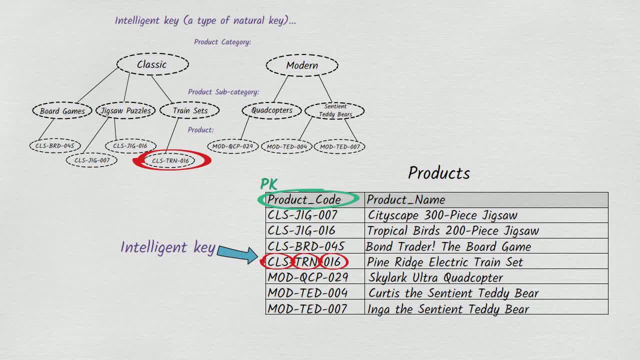 The product code is an intelligent key. An intelligent key is a natural key made up of multiple parts stuck together, with each of those parts having a meaning of its own. There are some pitfalls involved in using intelligent keys, Because an intelligent key has meanings built into it. 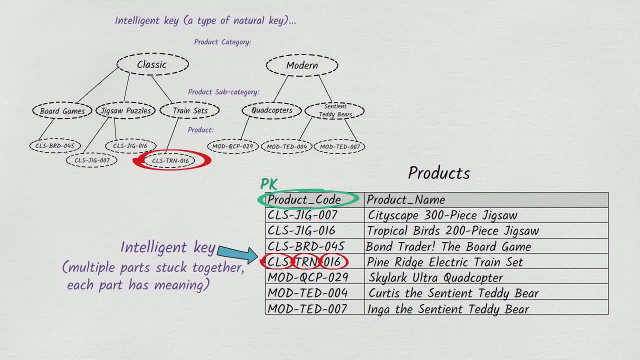 people might start to rely on being able to interpret it. People might start to extract those meanings from the key value. For example, people might devise reports that show product sales by product subcategory And to accomplish this they might rely on being able to recognize the product subcategory from the middle component of the product code. 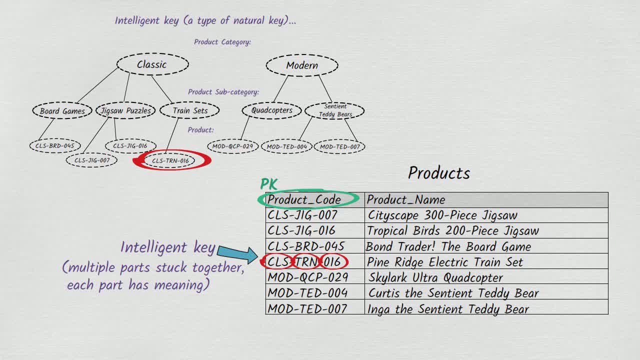 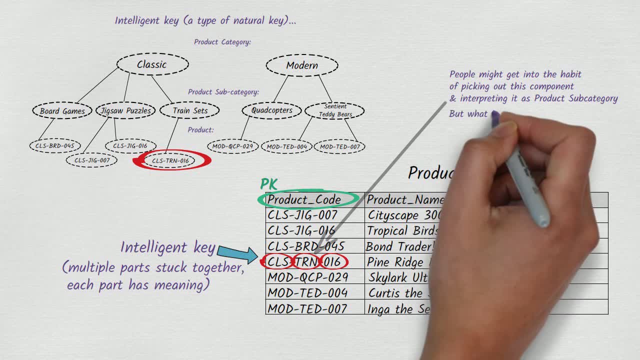 the part of the product code that has values like jig for jigsaw, BRD for board game, and so on. This is a very risky approach that will stop working if the company ever changes the format of its product codes. No one should ever assume that the product subcategory is a key. 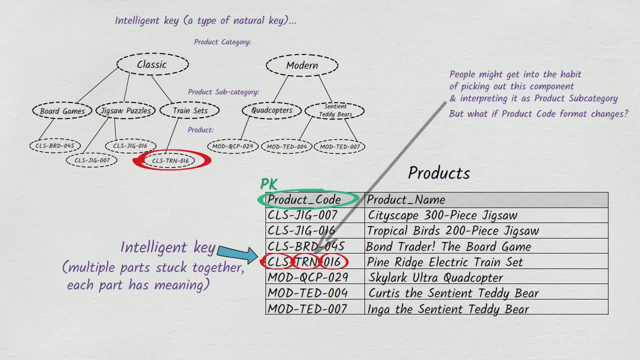 The product subcategory can be extracted from the product code. Instead, the product subcategory should be recorded explicitly in the database in its own column, And people should be encouraged to make use of that column. Another awkward thing about the intelligent product code is that it's not clear what's supposed to happen to it when products are re-categorized. 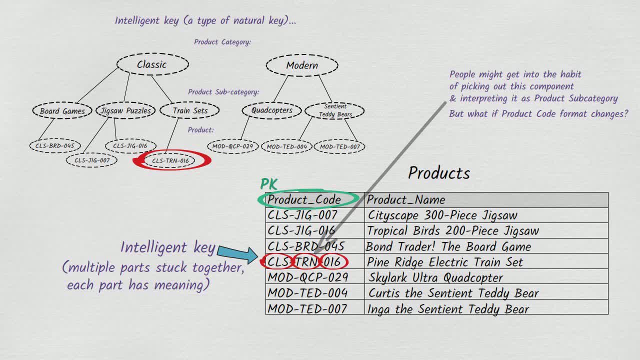 At the moment, all product codes start with either CLS or MOD, because all products are deemed to be either classic or modern. But what if the company doesn't have a product subcategory? What if it decides to stop categorizing its products as classic and modern? 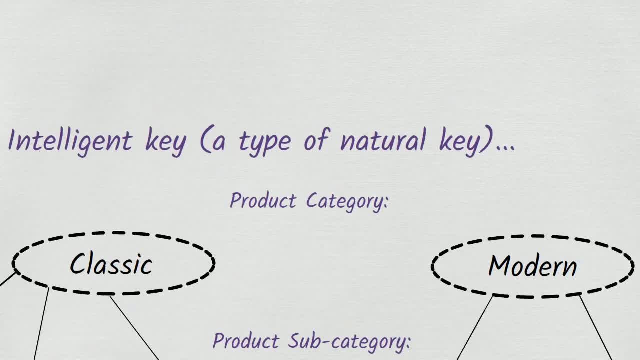 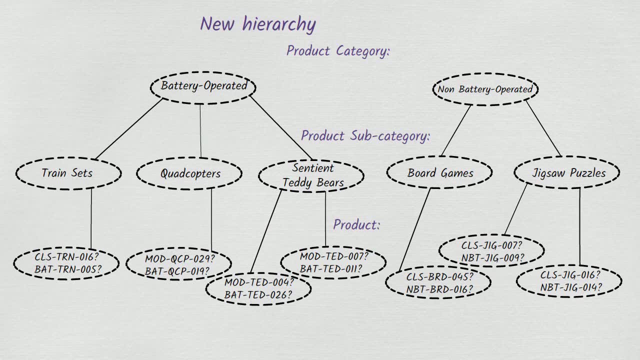 What if they decide to start categorizing products instead as battery-operated and non-battery-operated? Then there's going to be a conflict between the current format of the product codes and the company's new scheme of categories. At the very least, it's going to cause confusion. 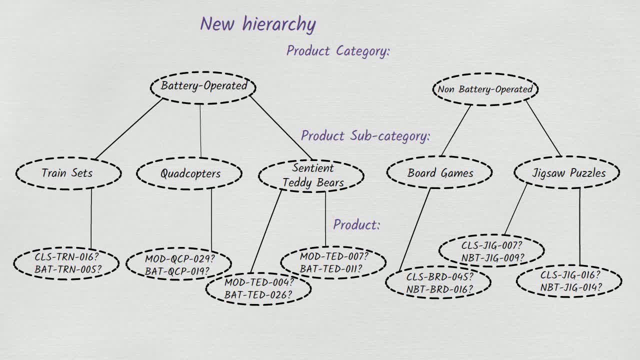 And in the worst case, it may require a large-scale update to the existing product codes in the database. None of this means that there should be a blanket ban on intelligent keys, but it does mean care needs to be taken when devising and using them. Intelligent. 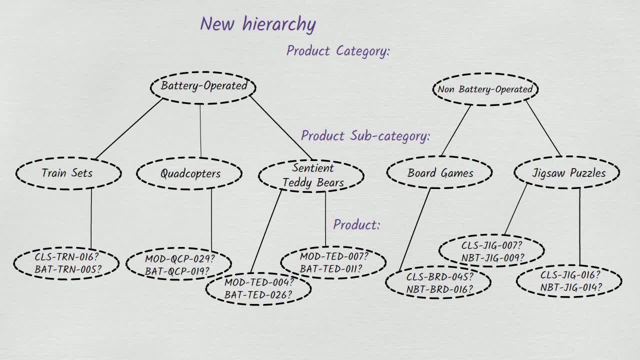 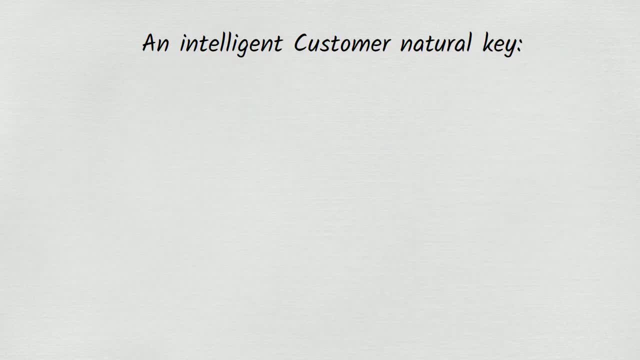 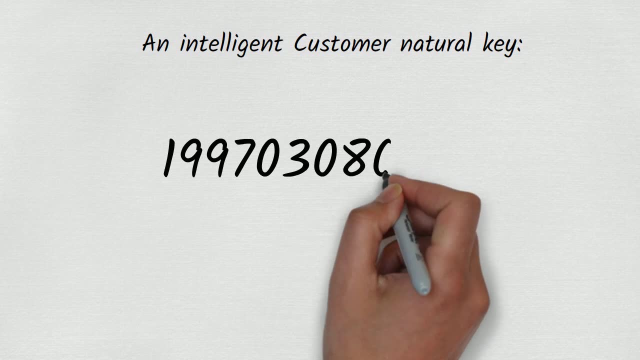 keys work best when the components that make up the key value really are essential to its identity. For example, we might imagine an intelligent customer natural key that's made up of the customer's date of birth followed by a sequence number, for example 1997 0308 0096.. The customer's date of birth is 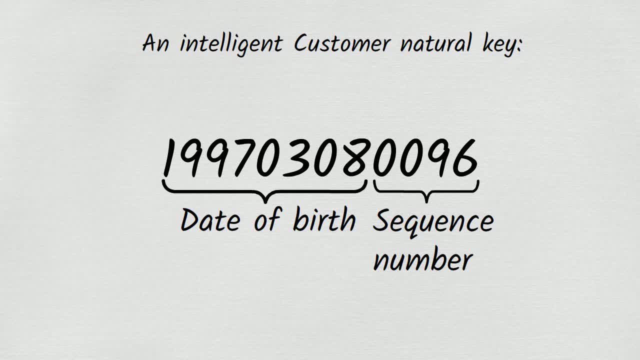 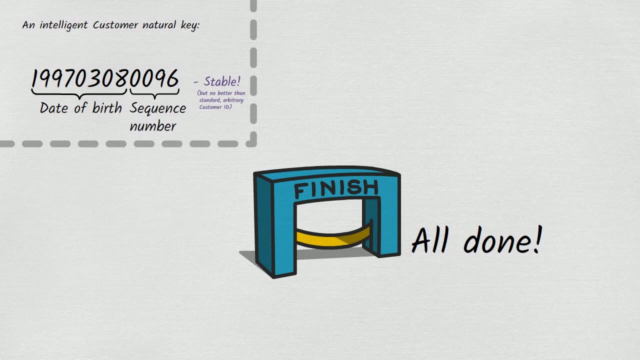 never going to change, so this is a stable identifier. It might not be any better than a completely arbitrary customer identifier, but at least it's unlikely to cause significant problems. This concludes our discussion of the different types of relational database keys. I hope you found this video helpful.